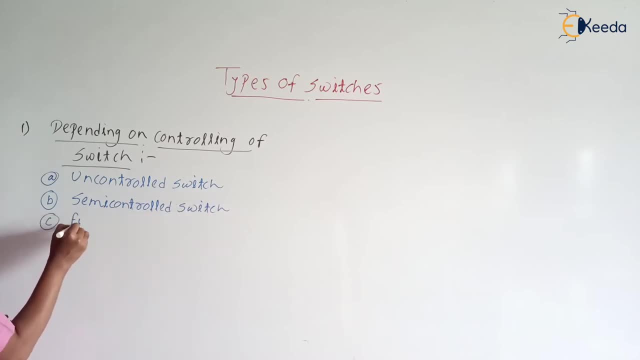 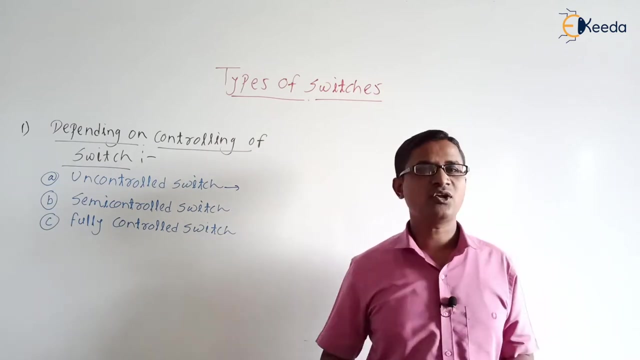 fully controlled switch. Okay, so these are the classification depending on controlling of the switch. Okay, so let us discuss first uncontrolled switch. The switch is said to be uncontrolled if it's either on state or off state, right, Sorry, if it's on state and off state. 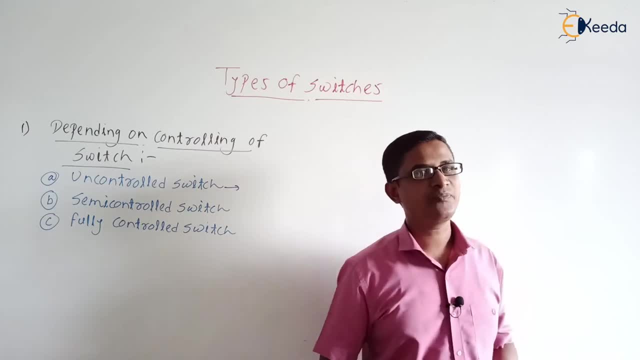 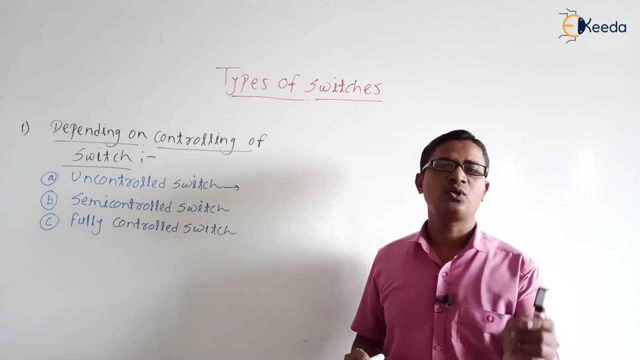 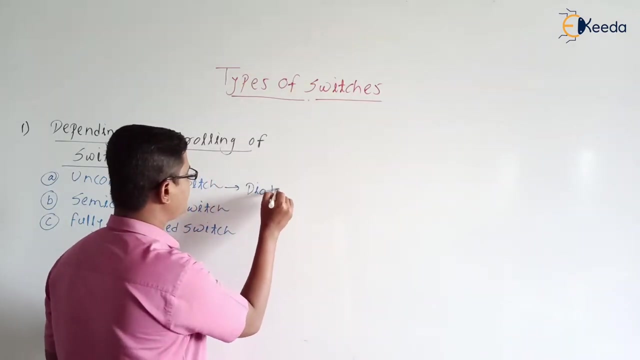 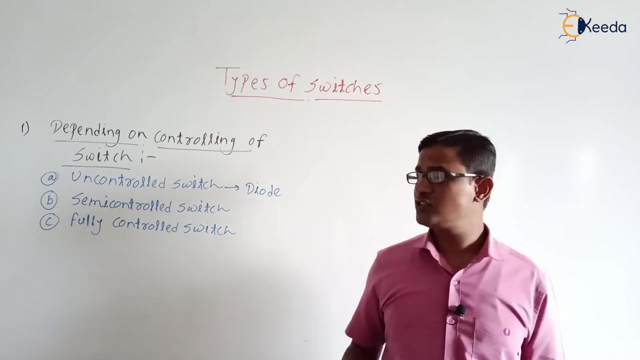 It cannot be controlled. The switch is said to be uncontrolled if it's on state as well as off state cannot be controlled by using the controlling signal or external signal. Okay, so one example of the uncontrolled switch: it is a diode, right, If you check the diode operation. the diode will be in the on state when the forward voltage appears across it, right? Otherwise, it will be in the reverse bias mode and it will be in the off state. Okay, so the diode will be in the on state when the forward voltage appears across it, right? Otherwise, it will be in the reverse bias mode and it will be in the off state. Okay, so the diode will be in the on state when the forward voltage appears across it, right? Otherwise, it will be in the reverse bias mode and it will be in the off state. Okay, so the diode will be in the on state when the forward voltage appears across it, right? Otherwise, it will be in the reverse bias mode and it will be in the off state. Okay, so the diode will. 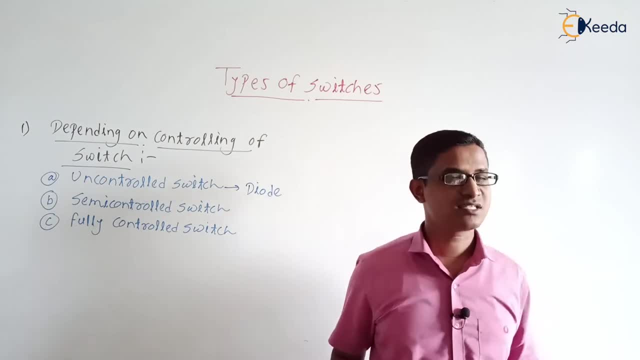 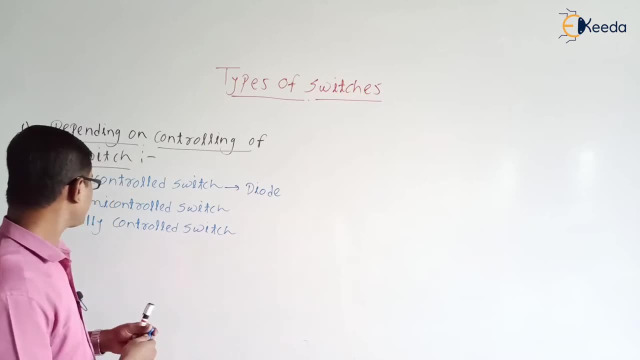 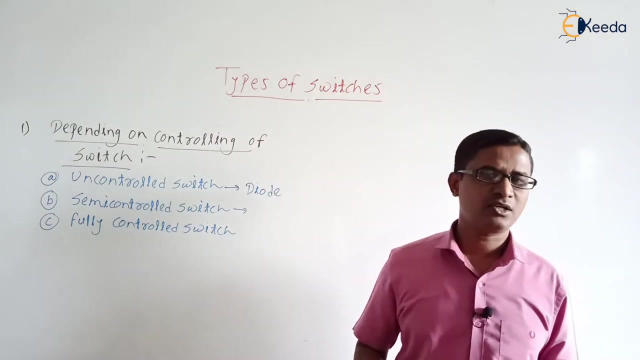 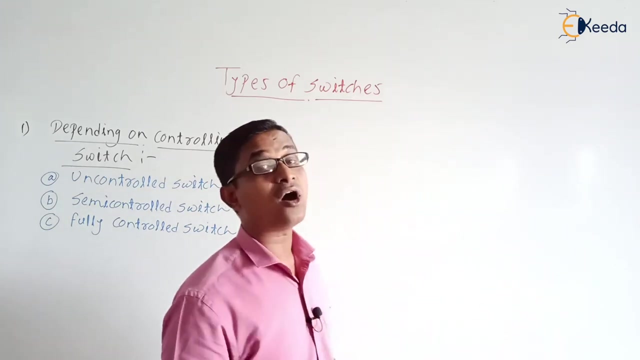 be in the on state due to the supply voltage. It is not due to the external signal. Are you getting the point right? So please don't get confused between external signal and the supply voltage. Okay. next, the semi-controlled switch. The switch is said to be semi-controlled. if it's either on state or off state can be controlled by using the controlling signal. Okay, either on state or off state can be controlled by using the controlling signal. Okay. one example is: 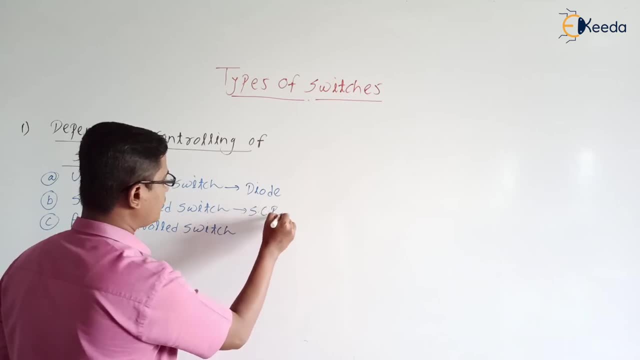 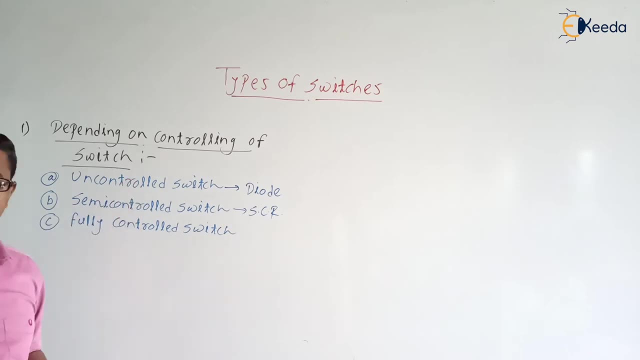 silicon controlled rectifier. right, Silicon controlled rectifier. Okay, if you know the SCR, definitely we're going to discuss in detail. Okay, so in the SCR, we can turn on the SCR by using the gate signal, but we cannot turn it off by using the gate signal. Is this clear? Okay, so SCR is a semi-controlled switch. Next, fully controlled switch. The switch is said to be fully controlled if it's on state as well as off state can be controlled by. 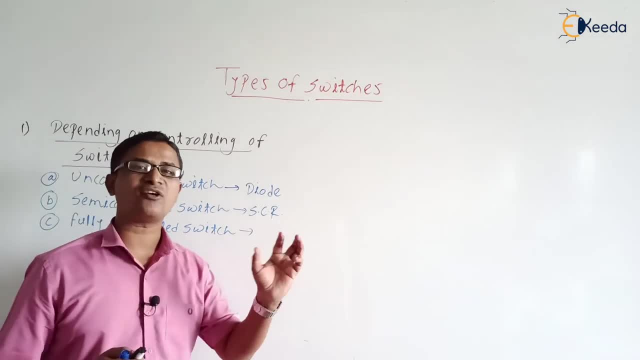 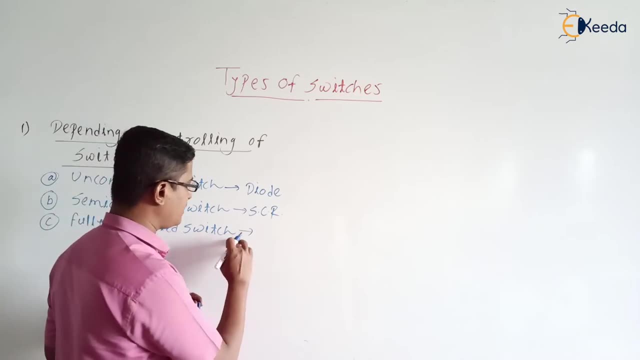 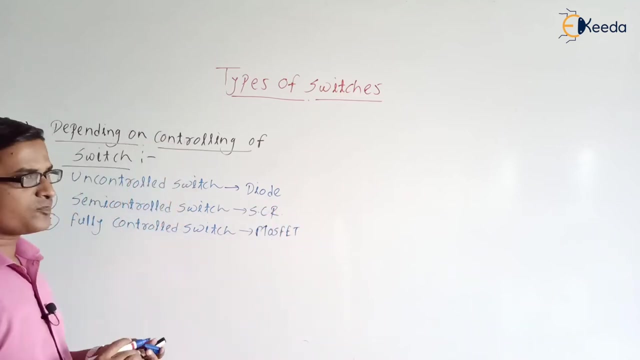 using the controlling signal. Okay means it's on state as well as off state can be controlled by using the controlling signal. Then the switch is said to be the fully controlled switch. Okay, example: yes, we're having the number of fully controlled switches- MOSFET, IGBT, BZT, etc. Okay, so this classification is based on the controlling of the switch. Okay, next second, depending on: 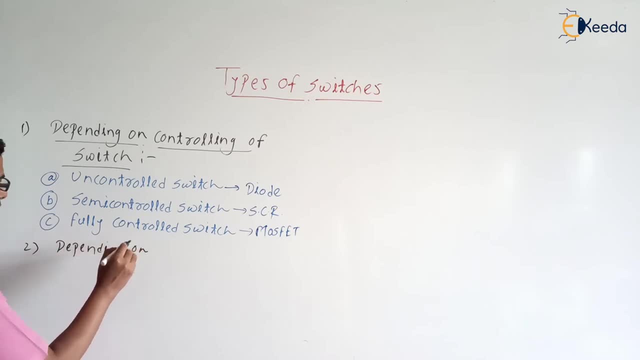 depending on direction of current, direction of current through switch, depending on direction of current through switch, during through switch, during on state, during on state. So here we need to understand, here we need to understand, need to concentrate the on state of the switch and the direction of the current flowing through. 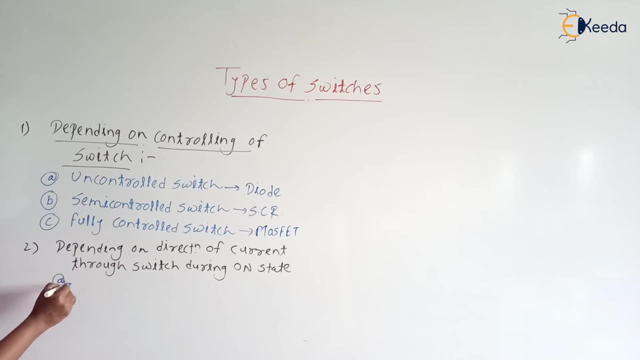 the switch. okay, so we are having the two types: one is a unidirectional switch, unidirectional switch and second one is a bidirectional switch. one is a unidirectional, second one is a bidirectional switch. okay, so so here we need to concentrate on on state of the switch as well as the direction of current 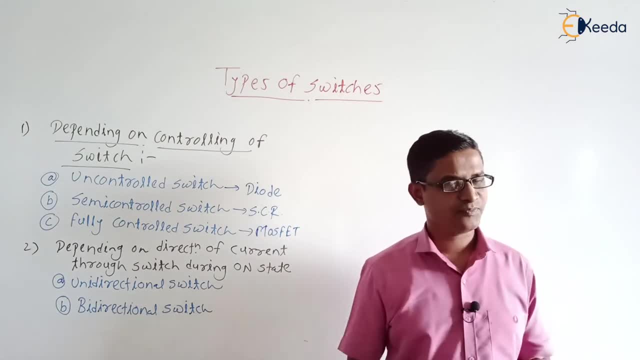 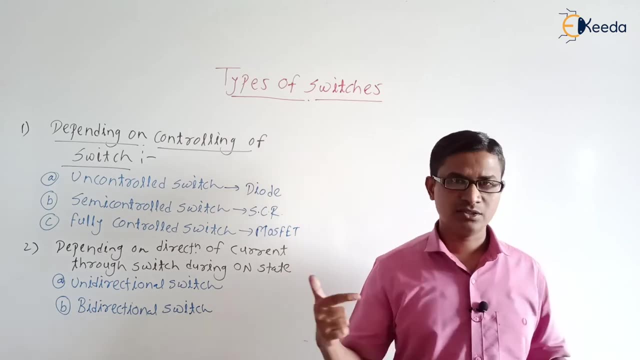 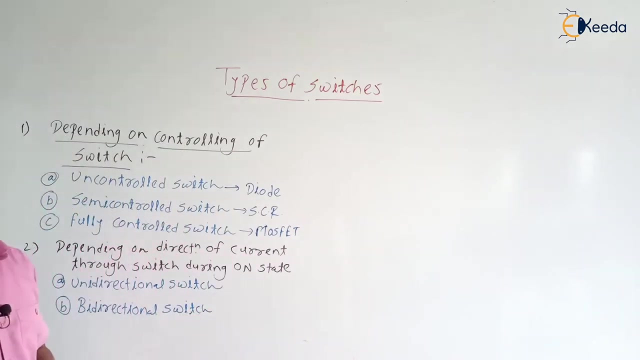 flowing through the switch. okay, the switch is said to be unidirectional. right, the switch is said to be unidirectional if it allows the current in only one direction through it during its on state. okay means the switch which is allowing the current in only one direction during its on state. 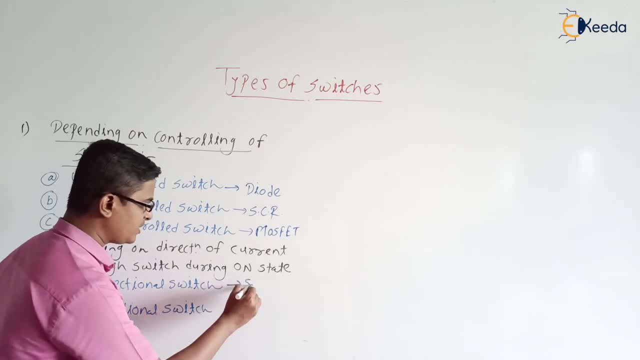 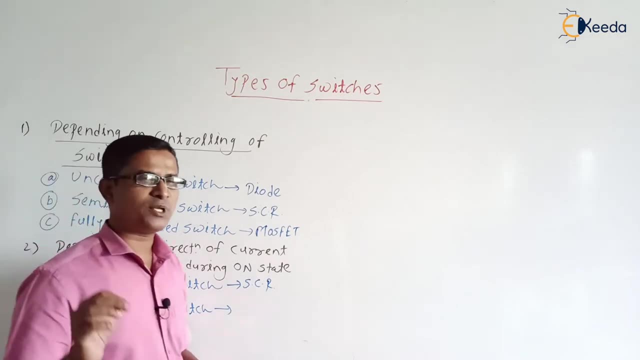 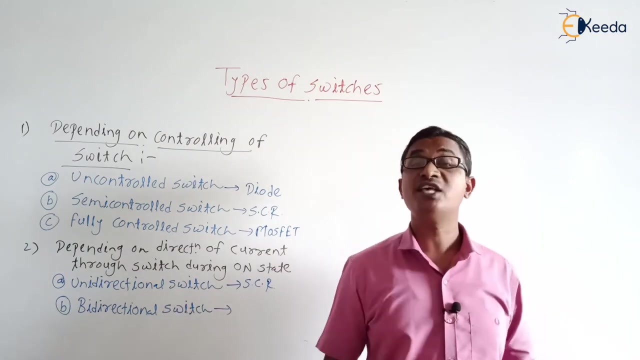 is known as the unidirectional switch. right, what is the example? scr is a example of unidirectional switch. okay, next, the bidirectional switch. the switch is said to be bidirectional if it allows the current in both the directions. that is, a forward as well as reverse, positive as well as negative during its 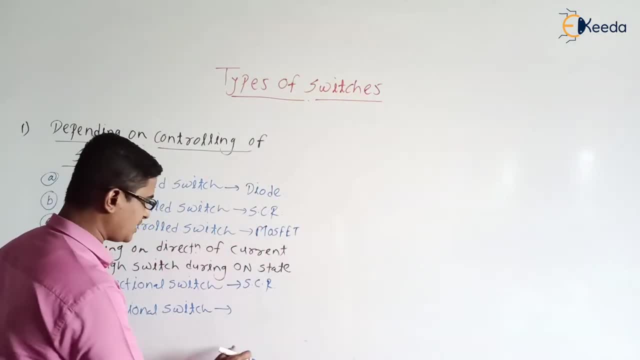 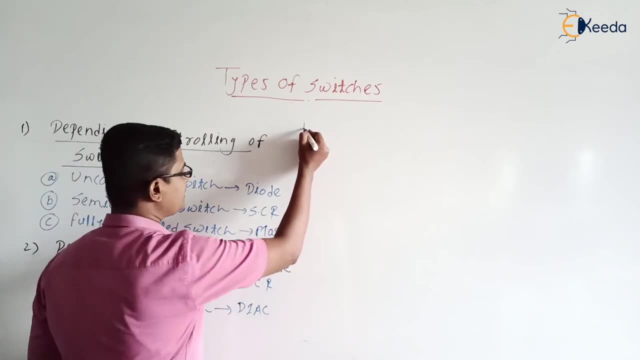 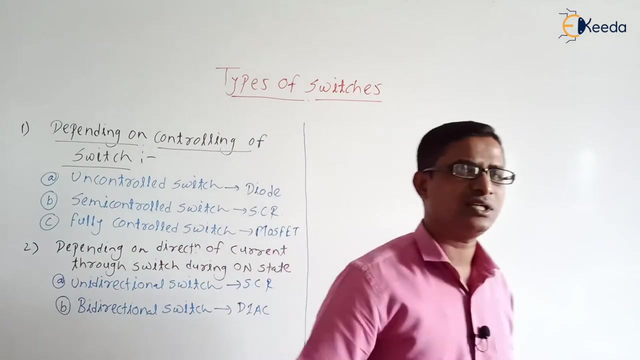 on state. okay. example of the bidirectional switch: yes, we are having the diac, we are having the triac, etc. okay, these are the examples of the bidirectional switch. right next related with a unidirectional bidirectional we are having, or we need to discuss the static operating points on vi plane also. okay, so they have asked the questions in the 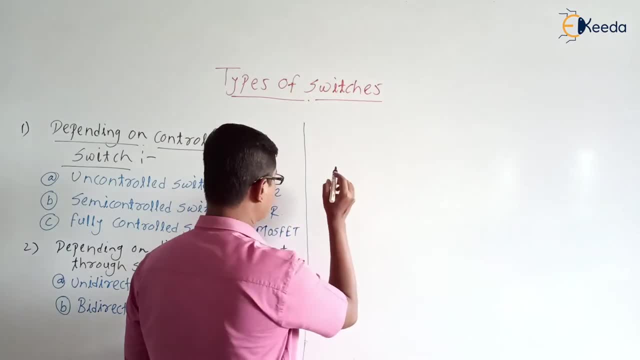 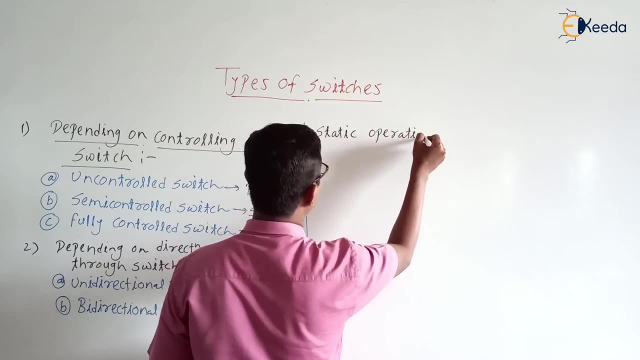 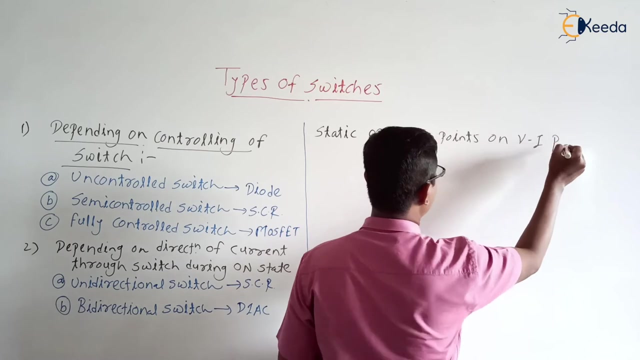 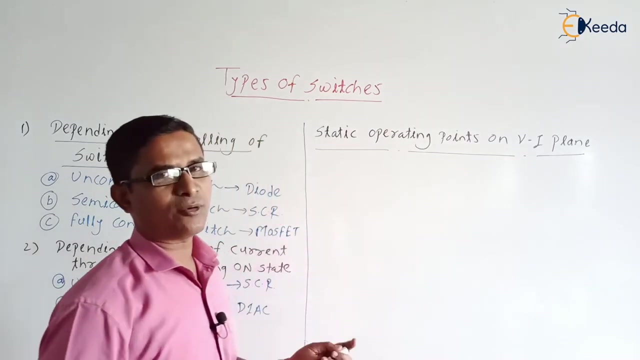 gate examination. this is a very, very important point. okay, so let us discuss static operating points. static operating points on vi plane. static operating points on vi plane. okay, so let us discuss one by one. okay, first, the static operating points position. if it is a unidirectional switch, perfect, I have. 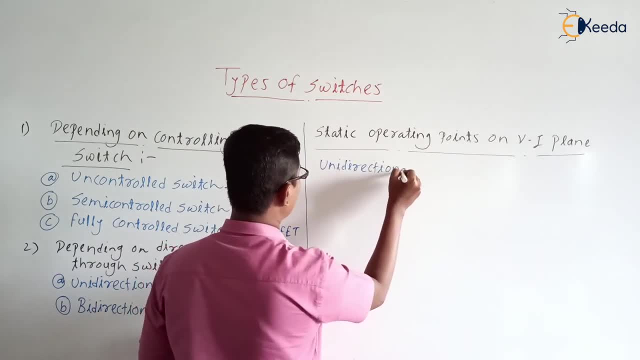 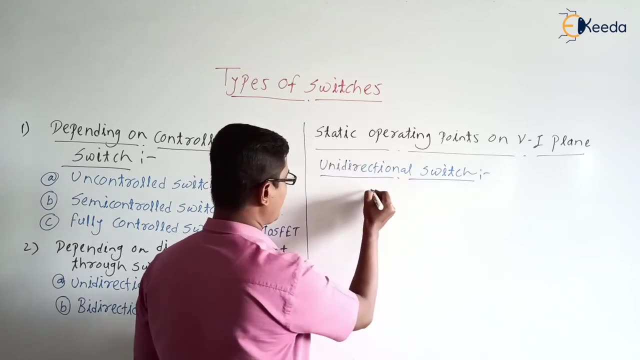 seen, there will be a static operating points like this. so by that we know there is one unidirectional switch. okay, if the static operating points is Büner's point, τη starting of stage is still positive, then it is a flat不會 передed. so what about diac? 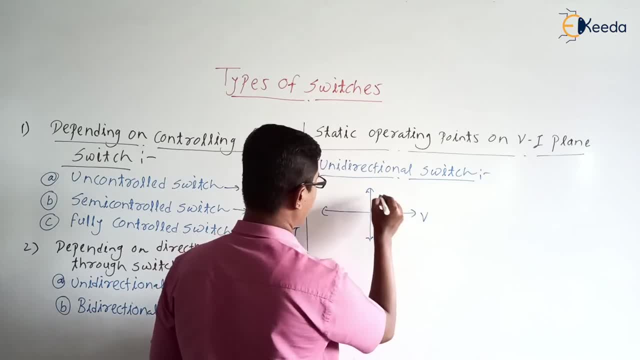 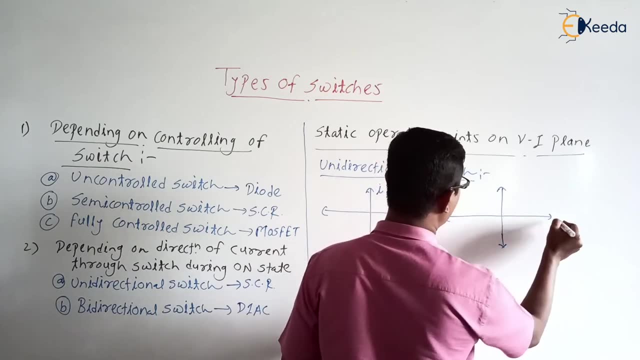 we have seen one combination like diac, the graph La zucchini T xi. justify like this. requesting Ł, we have your first input. we have a Noo's in that right. qualification points of vi relates to our vegetation. where, with the static operating point on VI plane for unidirectional switch for unidirectional switch? Yes, For unidirectional switch for unidirectional switch. where will the static operating points during the bi-directional switch is during the unidirectional switch and bidirectional switch? yes, the switch Is in the on state. 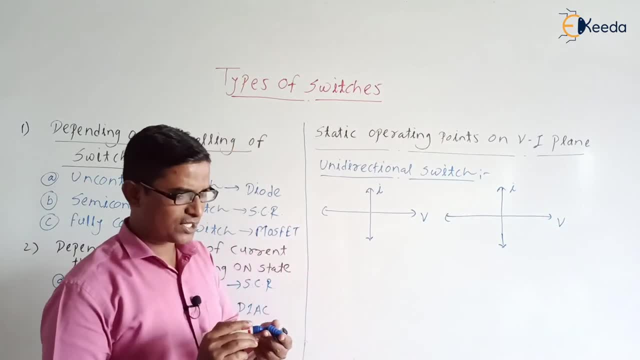 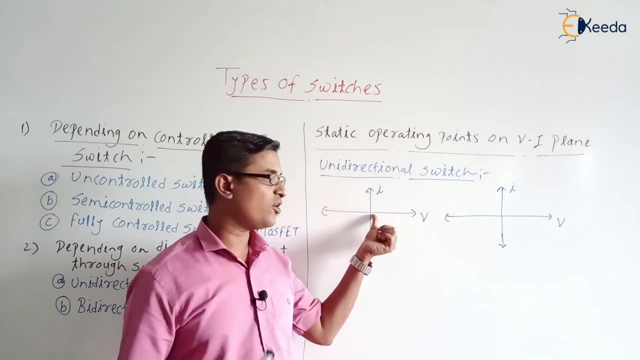 state only. okay. so when the switch is in the on state, what is the voltage across the switch? voltage across the switch is zero. okay, so voltage across the switch should be zero. so operating point will either lie on the positive i axis or negative i axis. are you getting the point okay? 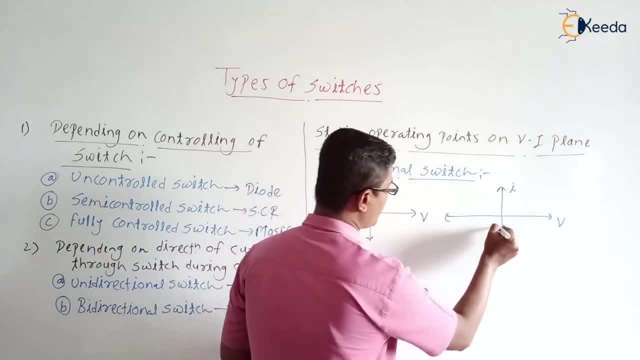 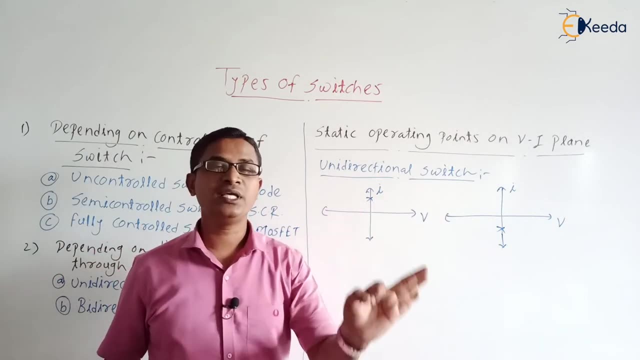 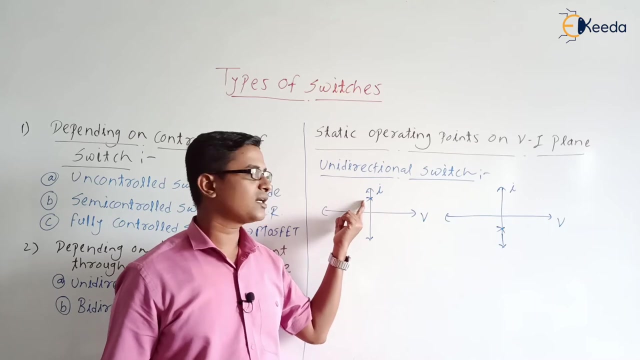 so here the static operating point is either here or here. are you getting the point right? these two indicates the static operating points for a unidirectional switch. is this clear? okay, so the switch is said to be unidirectional, right? so if you check the corresponding to this point, 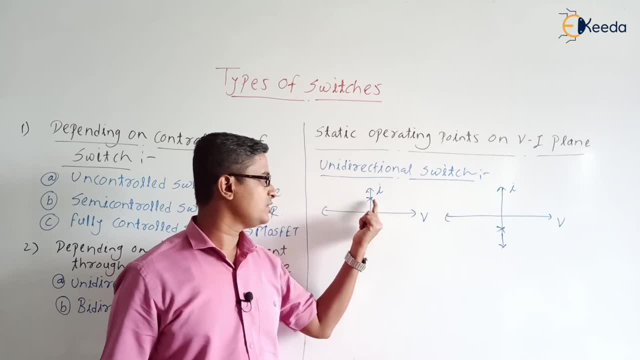 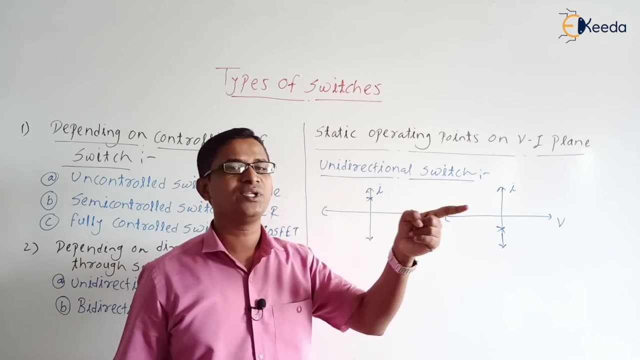 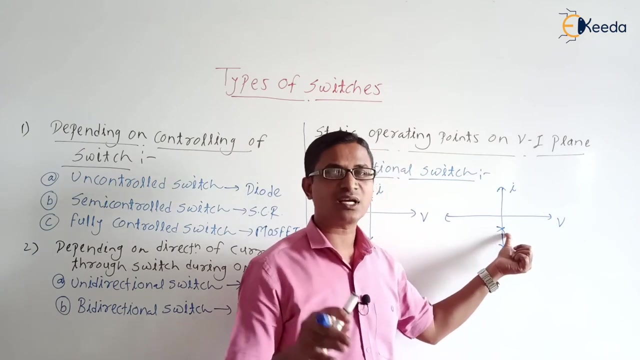 corresponding to this operating point. what is the voltage? voltage is zero. what is the current? current is positive means. the meaning is: this switch is allowing the current in only positive direction or forward direction. okay, next, corresponding to this point: what is the voltage? voltage is zero, but what is the current? 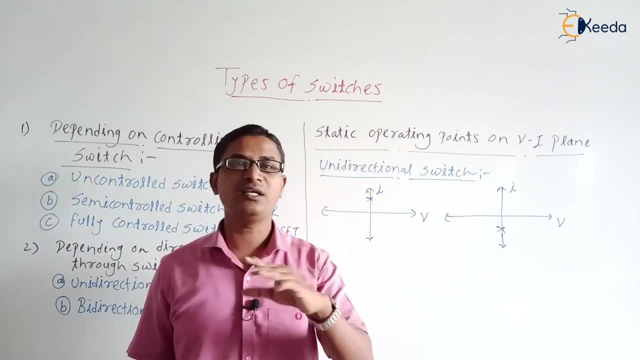 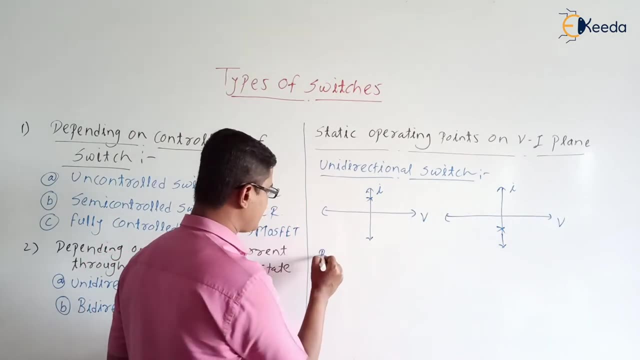 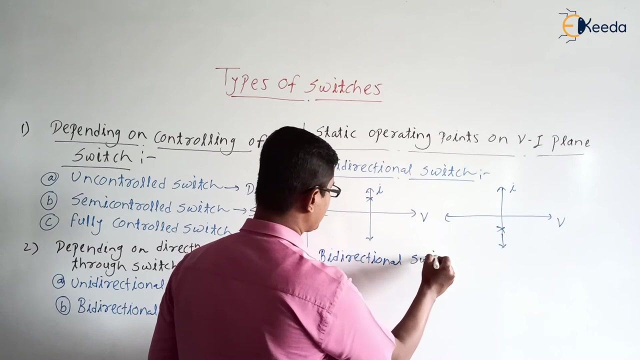 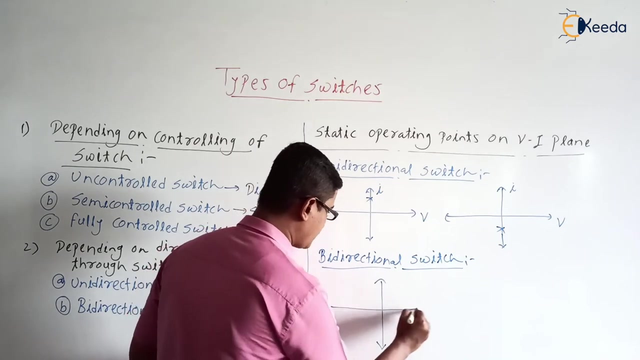 current is negative, the meaning is the switch is allowing the current in negative direction or in the reverse direction. okay, next let us discuss the static operating points for bidirectional switch. for bidirectional switch: for bidirectional switch: okay, now, as we know, for the bidirectional switch, yes, the switch allows current in both the directions, right? 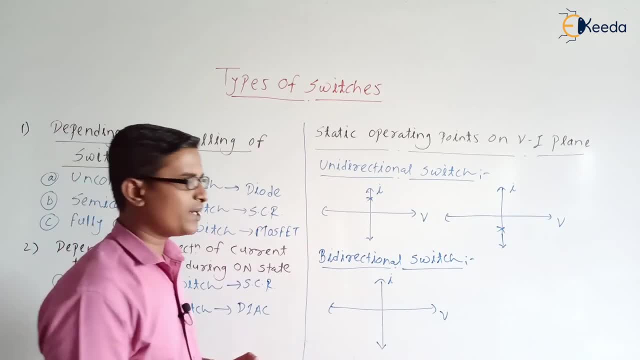 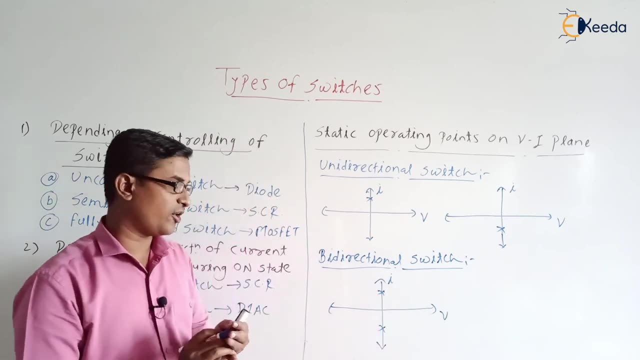 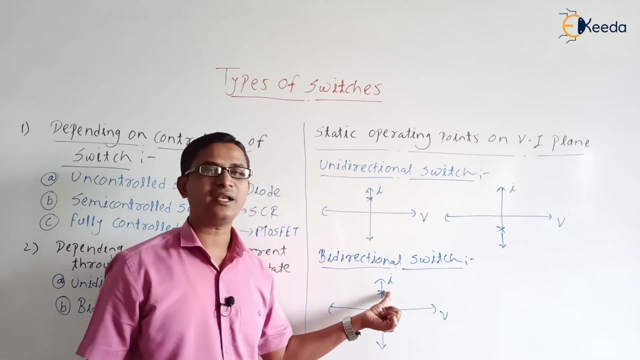 switch allows current in both the directions. so where you the static operating point? yes, as the switch is in the on state, so voltage should be zero. so point will be either here or here, right? sorry, point will be here as well as here. is this clear to all? okay, so, corresponding to this point, the voltage is zero, right, and current is positive. 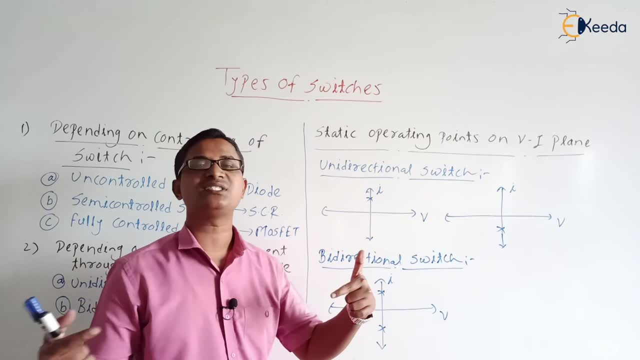 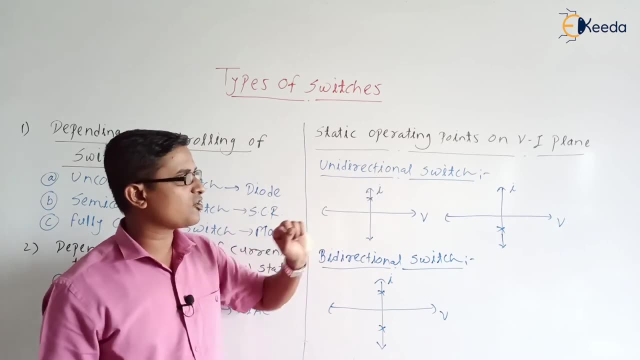 corresponding to this point. the voltage is zero, current is negative means the switch is allowing the positive current as well as negative current, forward current as well as reverse current. is this clear? so this is about the static operating point on vi plane. okay, in the gate examination they have 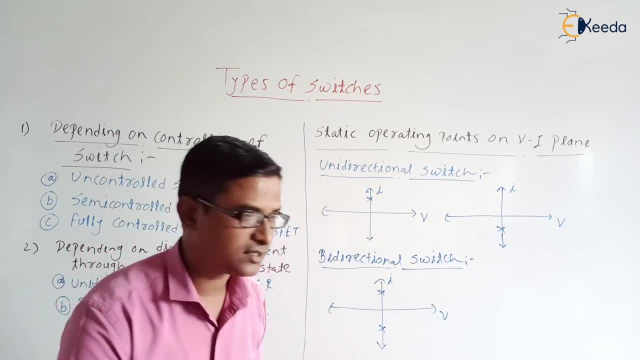 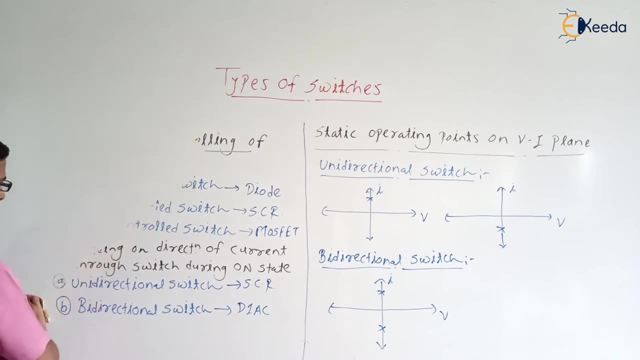 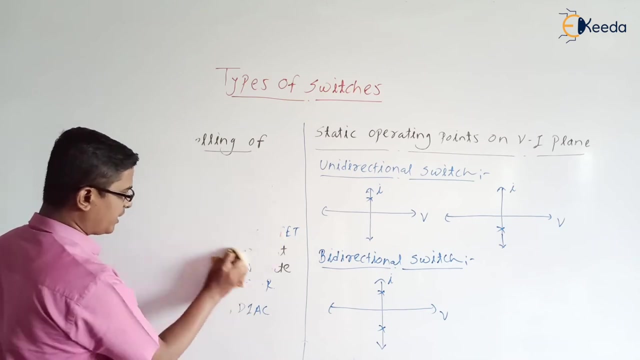 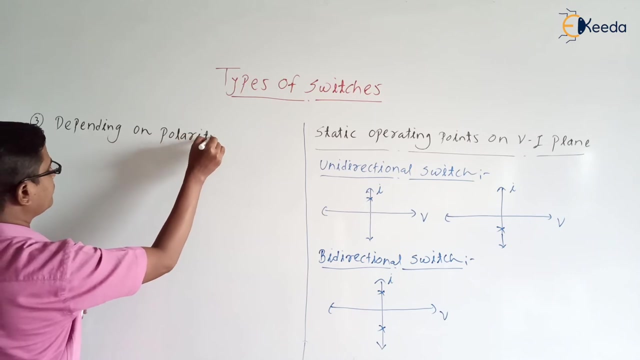 asked the questions based on it. right next, the third classification, or the third type, is depending on polarity of voltage blocked by the switch during its off state. okay, we are going to discuss third classification depending on on: depending on polarity of voltage. polarity of voltage blocked by switch. polarity of voltage blocked by switch. 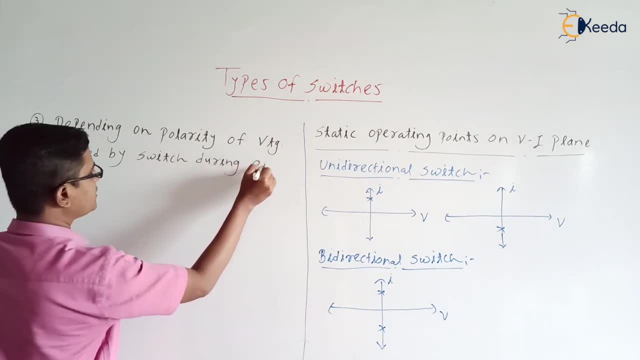 during off state. very important dinero. very important during off state. very important during off state. so here we need to concentrate on off state as well as the polarity of voltage across the switch: right polarity of the voltage across the switch. okay, so we are having the two types. one is 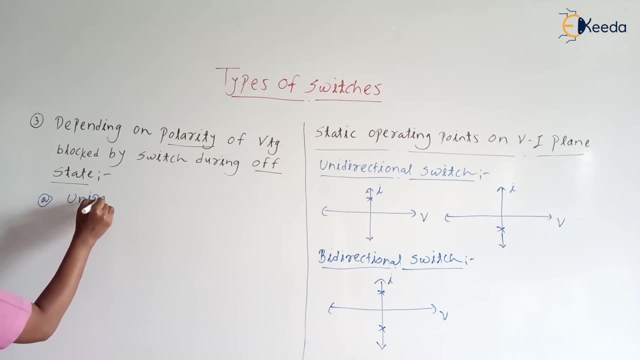 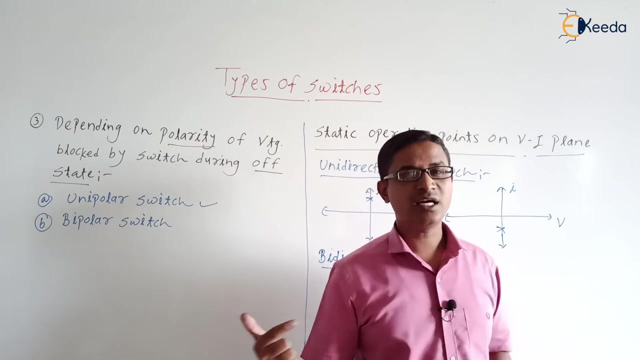 unipolar switch and second one is a bipolar switch. unipolar and bipolar switch. okay, so let us discuss one by one. unipolar switch: the switch is said to be unipolar if it blocks either forward voltage or reverse voltage, if it blocks either forward voltage or 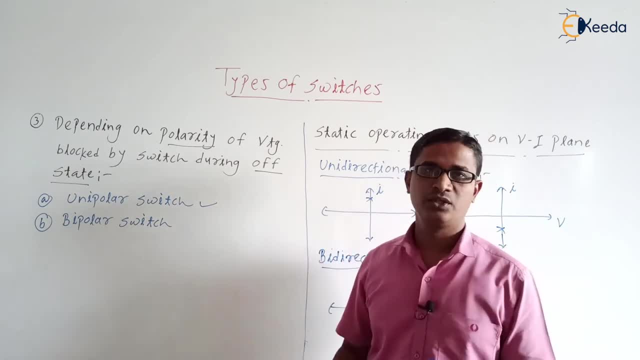 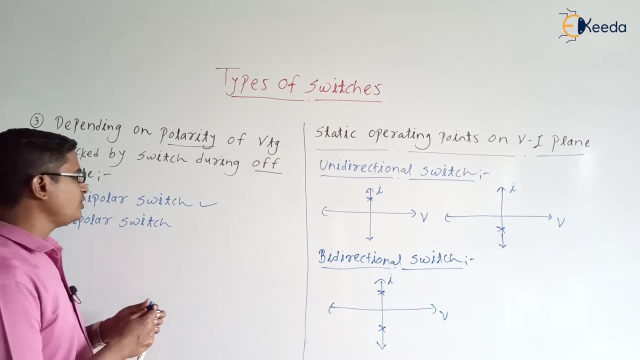 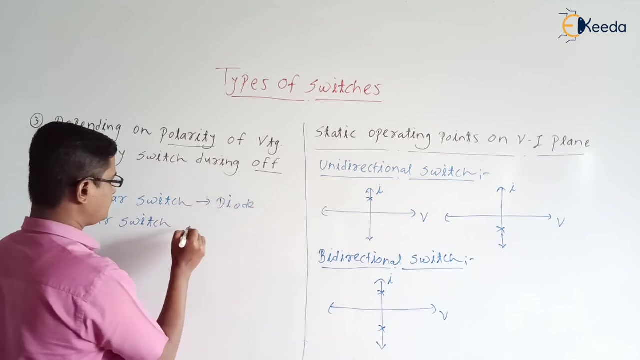 reverse voltage during its off state during its off state. okay, so it is blocking either forward or reverse voltage. okay, so one example of unipolar switch right example of unipolar switch: diode: diode. as we know, you might have heard the diode when it is in the forward bias mode. 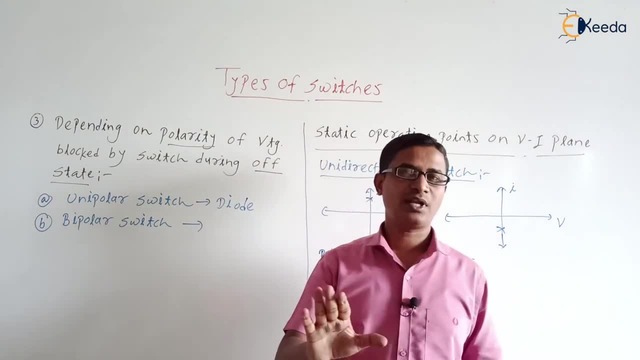 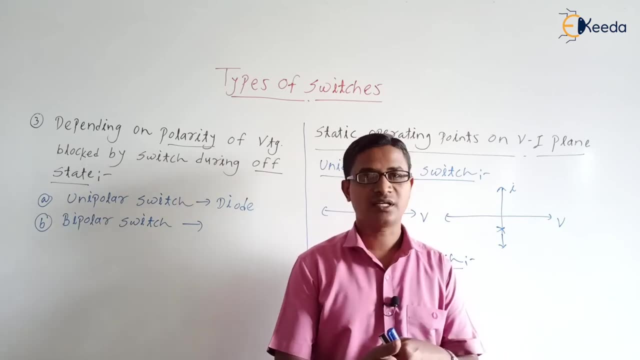 whether the diode blocks the voltage. no, right. when diode is in the forward bias mode, the diode starts conduction. so diode is conducting. means what diode is acting as a short circuit. so what is the voltage across the diode? voltage across diode will be zero. okay, means diode is not blocking. 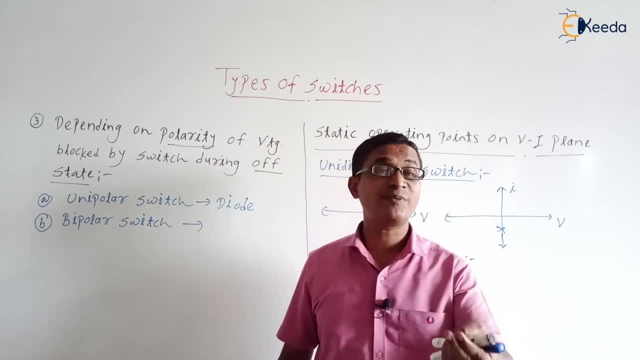 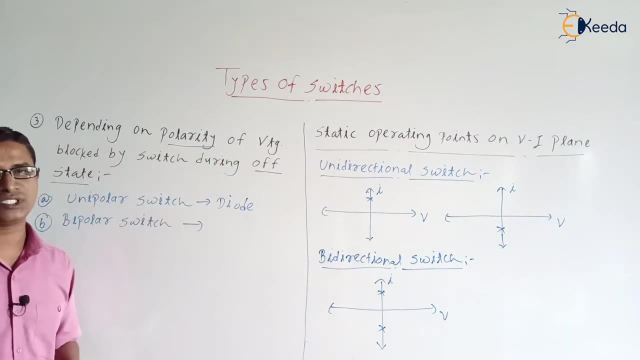 the voltage when it is in the forward bias mode, but when it is in the reverse bias mode, the definitely the diode blocks the voltage right. so diode is blocking only negative voltage. that's why it is a unipolar switch right. next one is a bipolar switch. thus which is 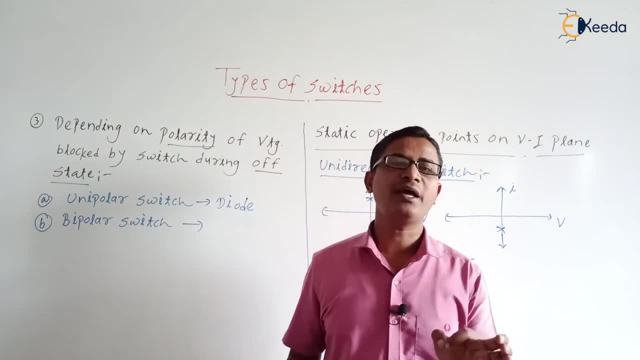 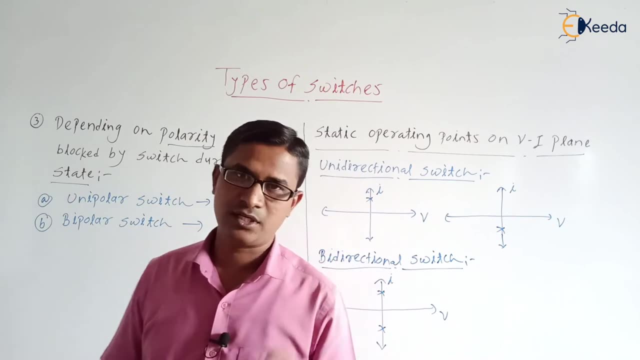 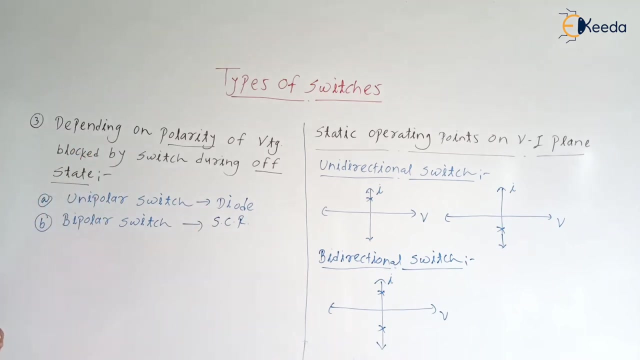 said to be bipolar if it blocks forward as well as a reverse voltage. okay, if it blocks forward voltage as well as a reverse voltage during its off state. during its off state. one example of bipolar switch: SCR. as here is an example now. bipolar switch: okay, we're going to discuss in detail what is the STR right and what areresаботable of bipolar switch. okay. 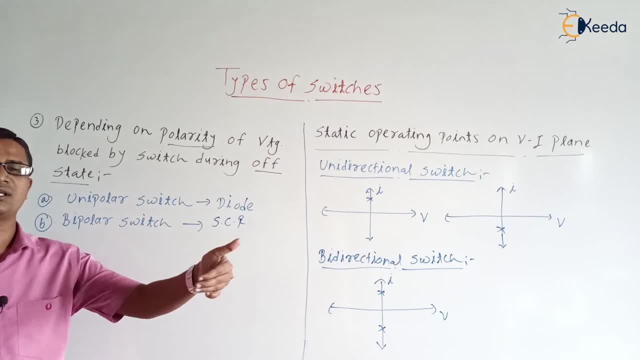 So here is the SCR. alguém muah brother program in a longвой, a port Korean bipolar switch. okay, now we're going to in detail what is the scr right and what are the characteristics? okay, at that time you will understand why it is a bipolar switch. okay, so before that, let us discuss static operating points. 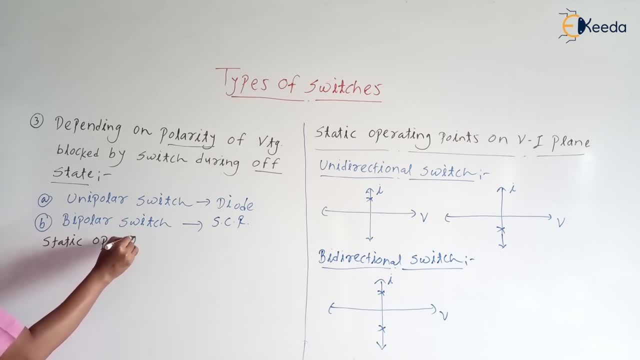 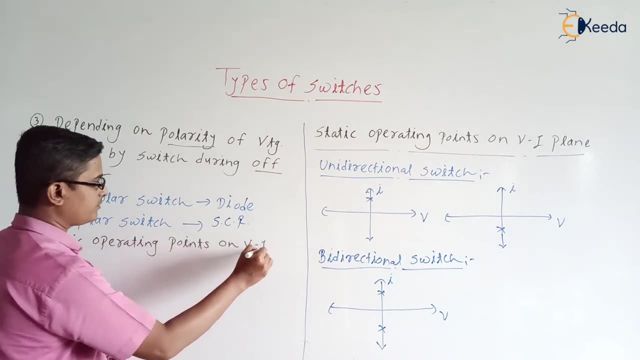 static operating points. static operating points on vi plane. on vi plane, right for unipolar and bipolar switch. for unipolar and bipolar switch: okay, so let us first discuss for unipolar switch. first one is for unipolar switch. okay, so for unipolar switch. as we know, 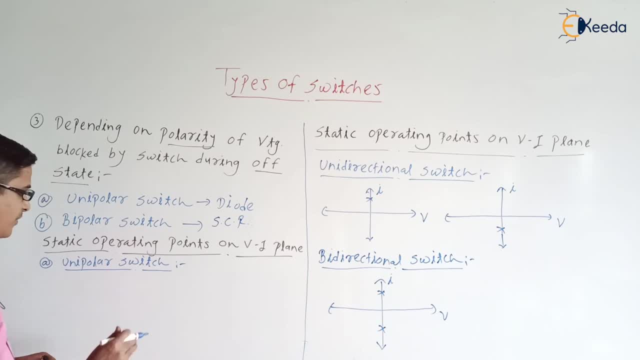 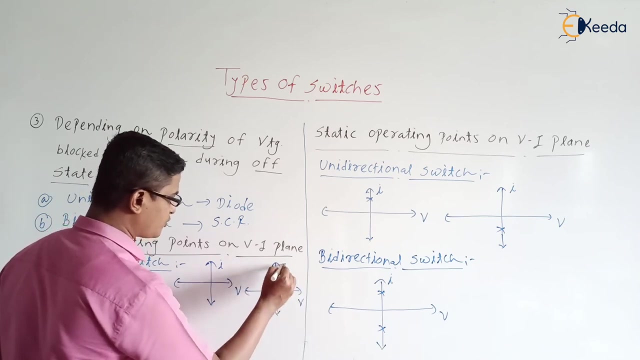 the switch. unipolar switch blocks either forward or reverse voltage during its during its off state. okay, so switch is in the off state. so what is the current voltage? current right. so when the switch is in the off state, what is the current flowing through the switch? current flowing through the